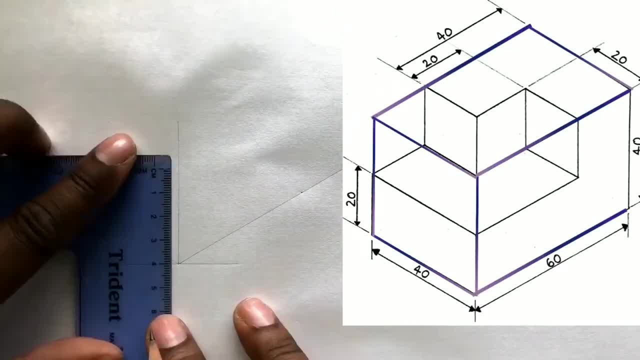 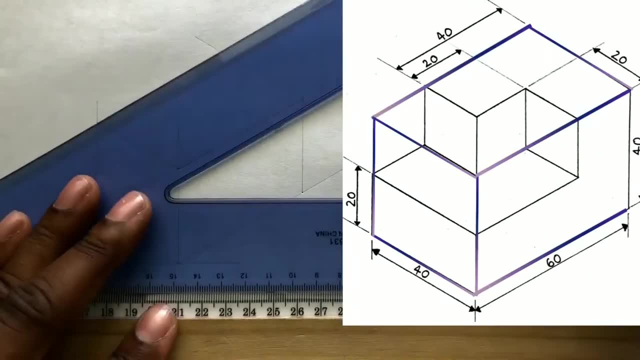 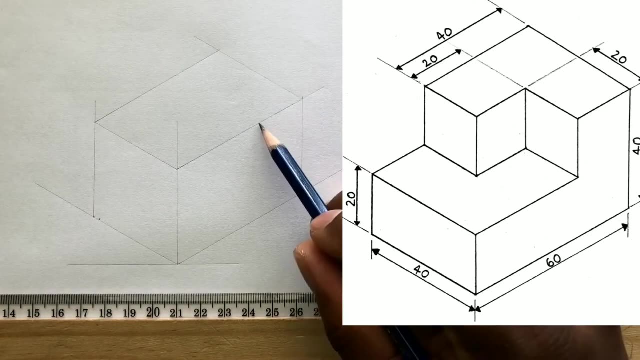 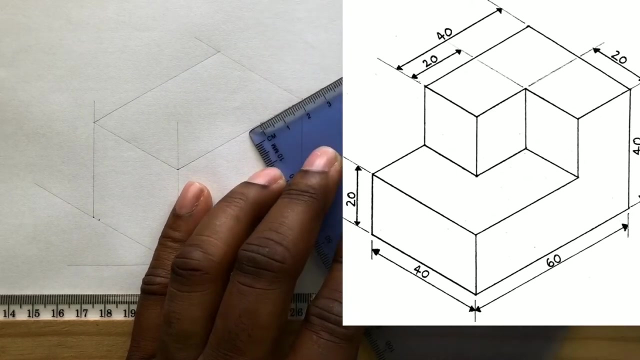 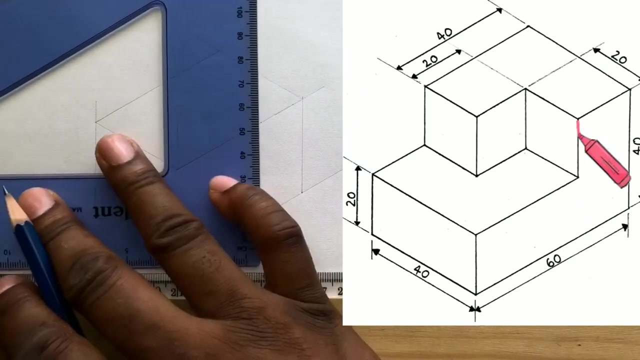 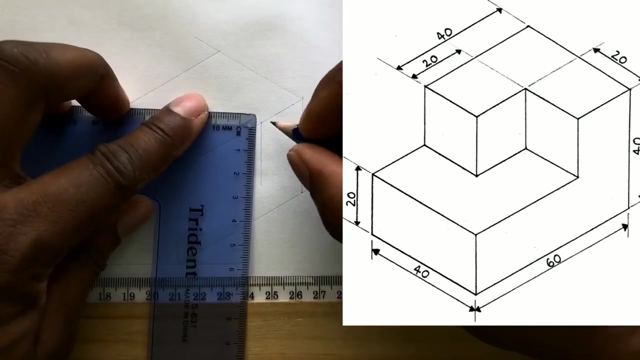 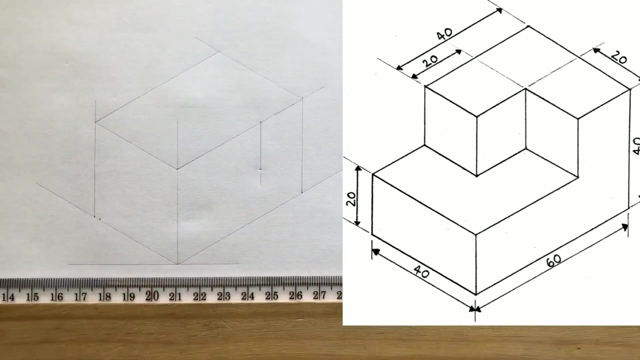 Now measure and identify 20 millimeters from this intersection on this line. Now draw a vertical line from this point in this direction. Measure and identify 20 millimeters from this intersection on this line. Now, from this point you identified, draw a horizontal line using your set square and your. 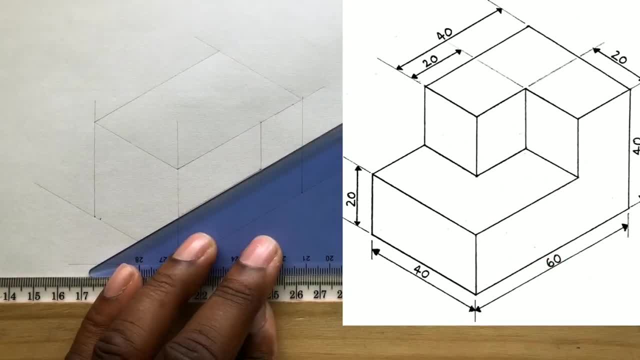 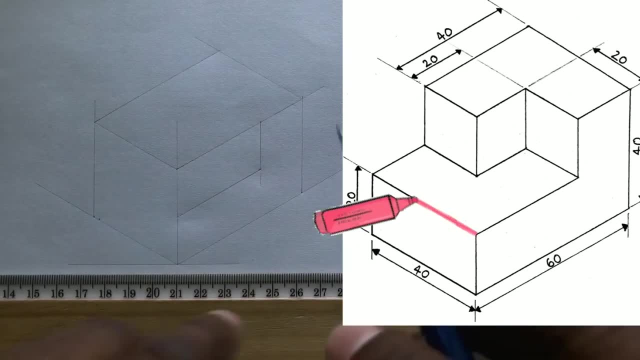 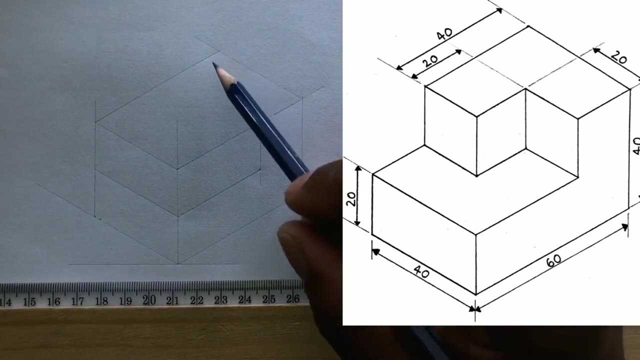 t-square in this direction. Also, draw a horizontal line from this intersection to the given dimensions. Now, from this point you identified, draw a horizontal line using your t-square in this direction. Now, measure and identify 40 millimeters from this intersection on this line, 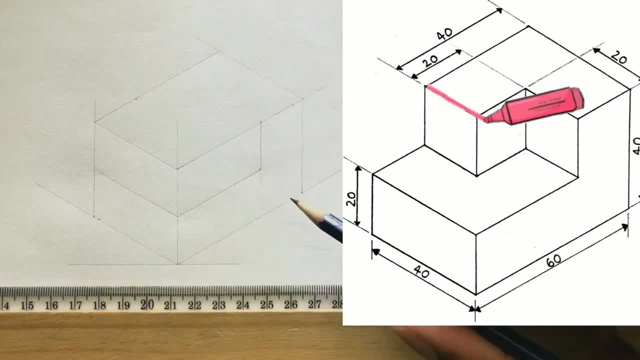 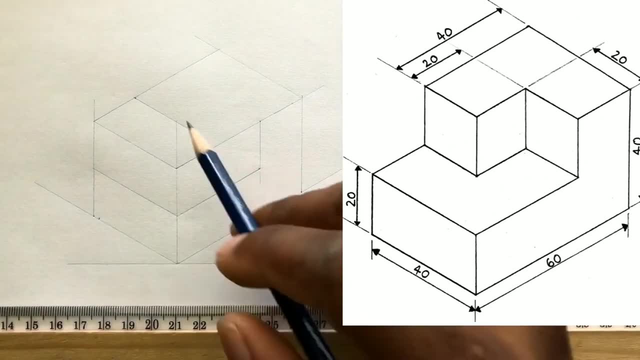 Now draw a horizontal line from this point in this direction. Also draw a horizontal line from this point in this direction. Now draw a horizontal line from this point in this direction. Also draw a horizontal line from this point in this direction. 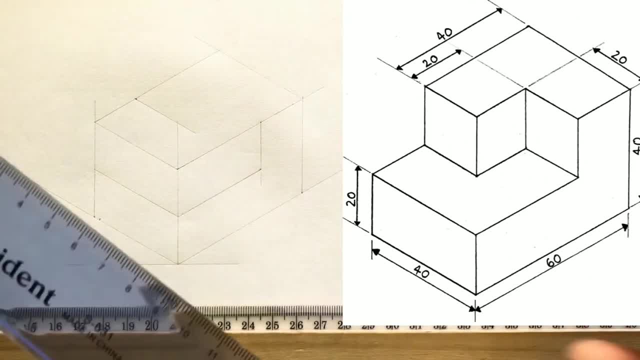 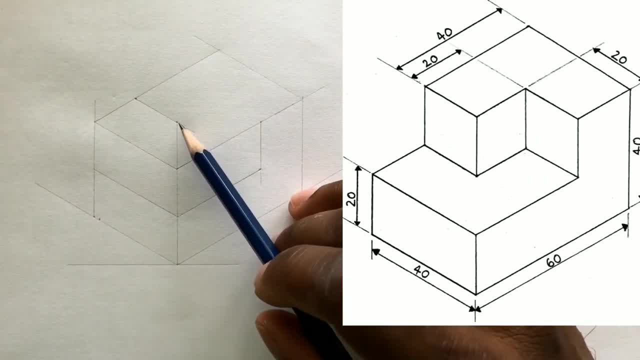 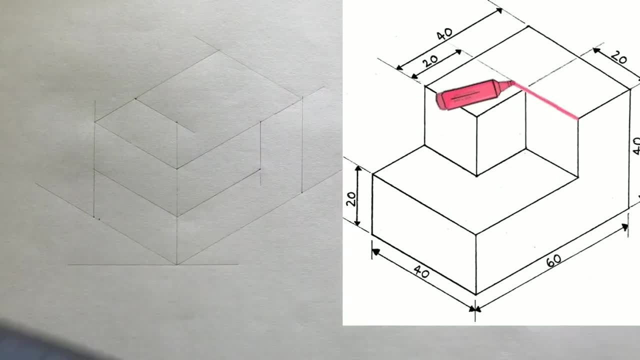 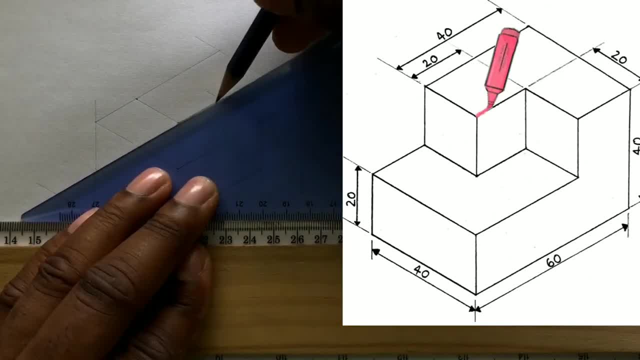 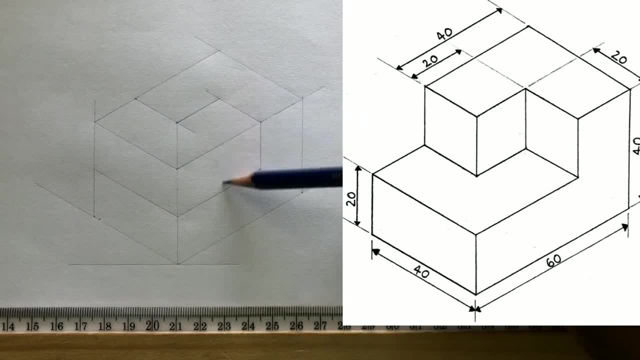 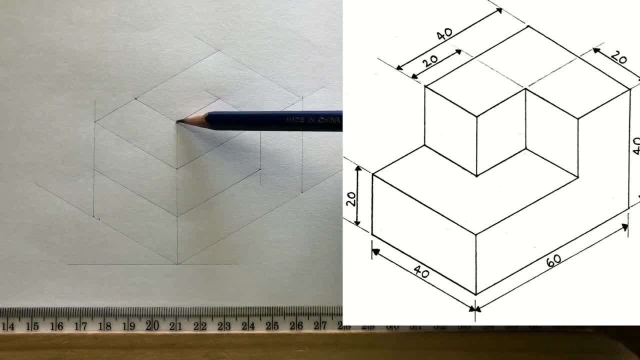 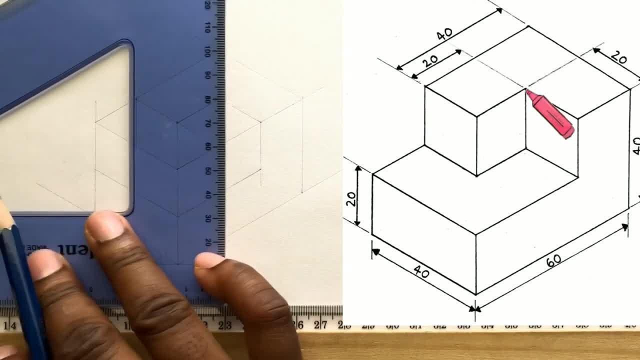 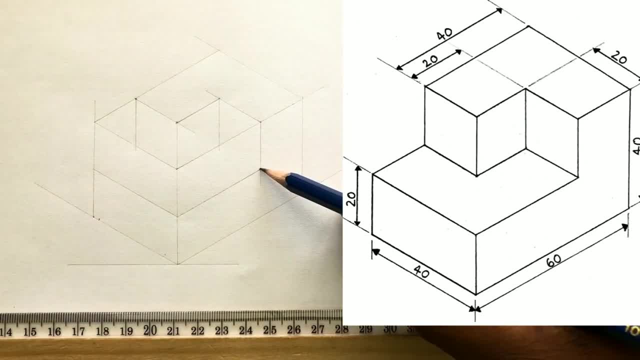 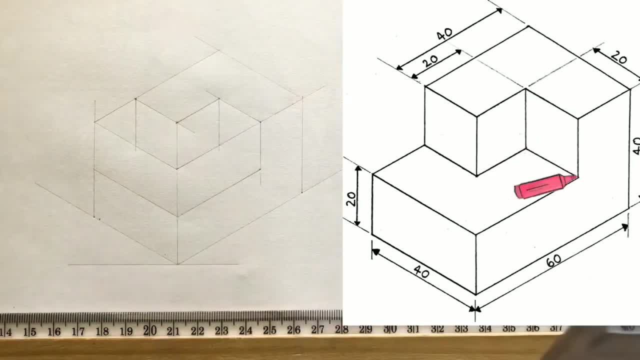 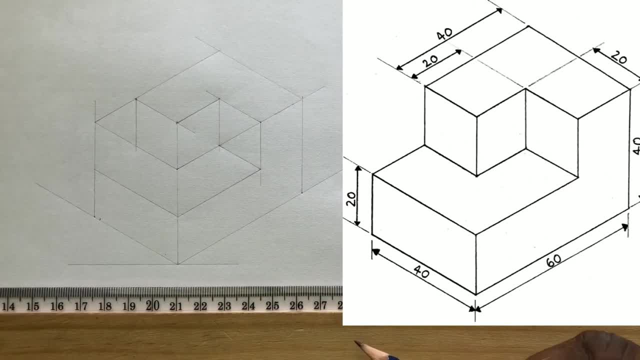 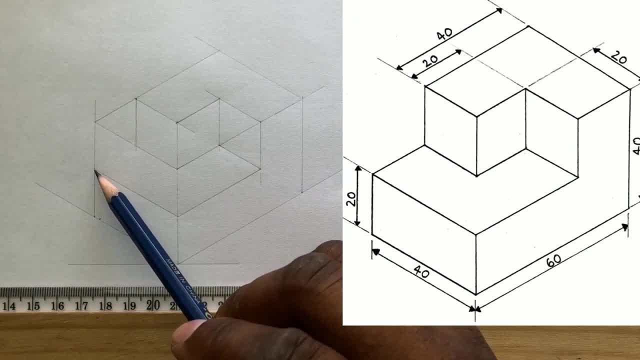 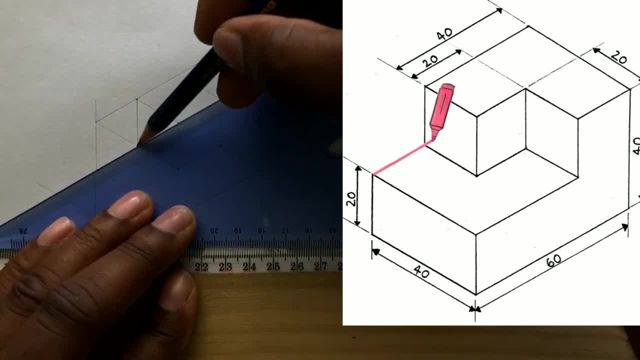 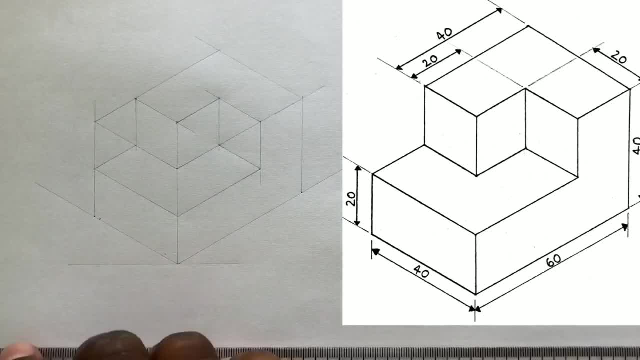 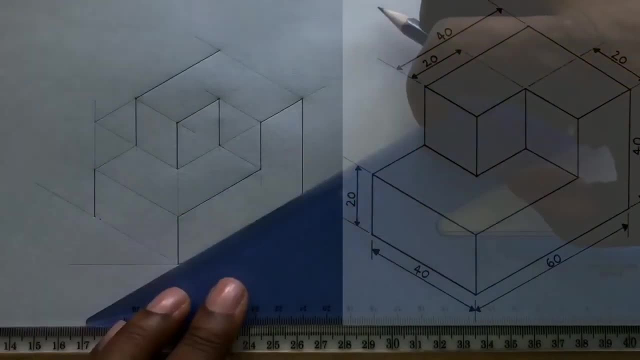 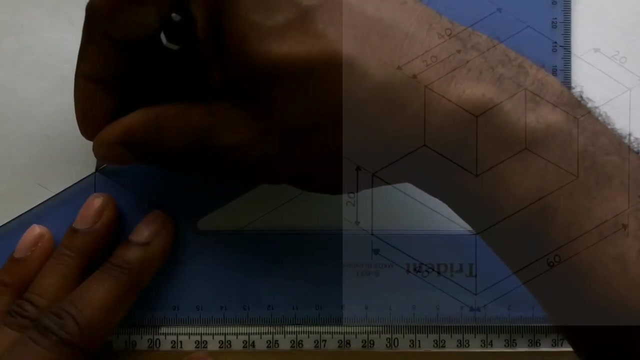 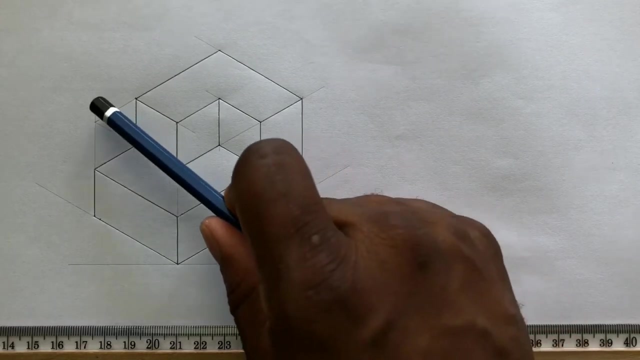 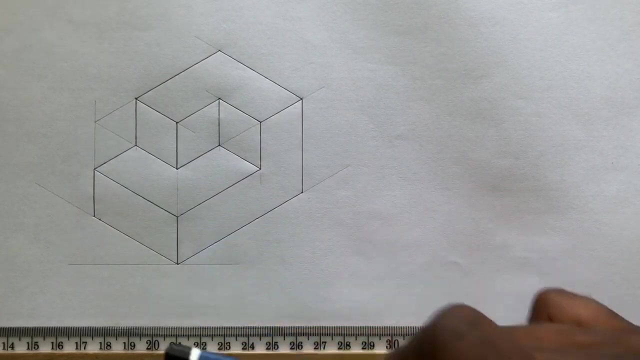 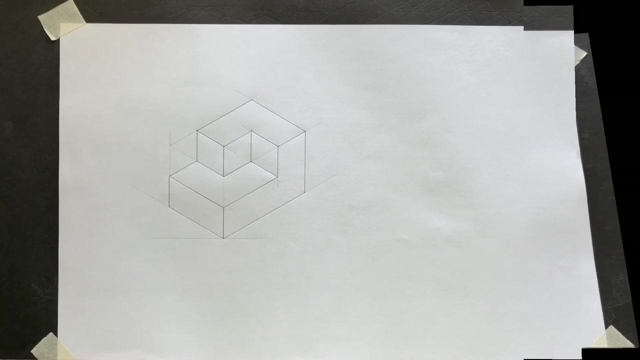 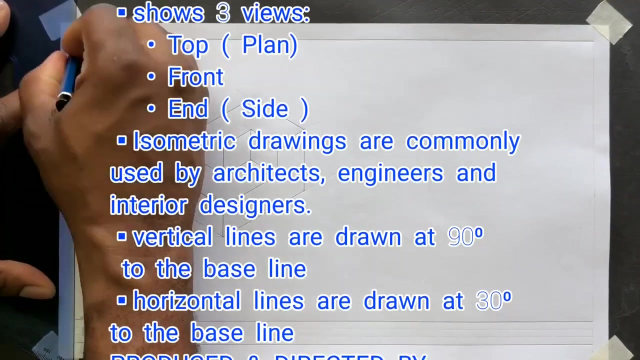 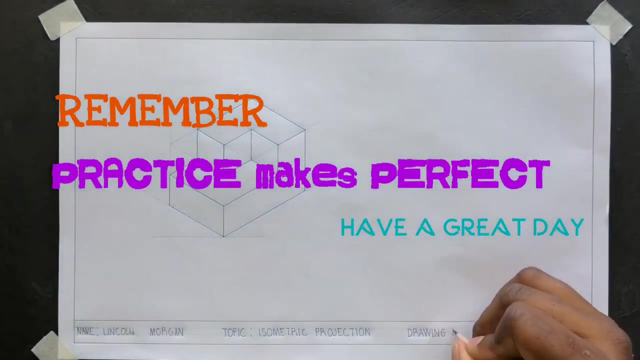 Also draw a horizontal line from this point in this direction. excellent, it was not so hard at all. now you realize that by just drawing an isometric rectangle you can easily draw more complex shapes. now go ahead, border your paper and complete your title block.